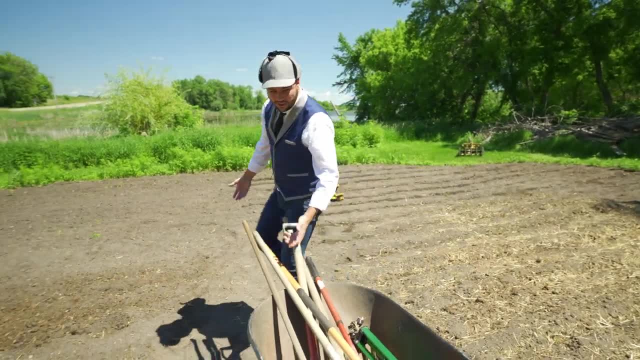 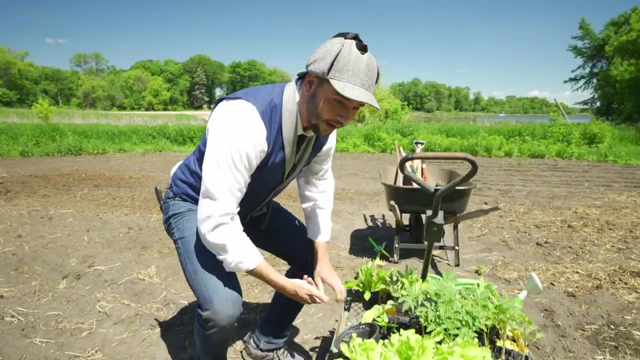 Those are all the tools that we're going to use to help us plant a garden. Well, hey, do you remember? in one of my earlier episodes we planted a bunch of seeds. Look at all of them. You know what I think? I'm going to bring in one of my friends, a junior inspector, to help us out. 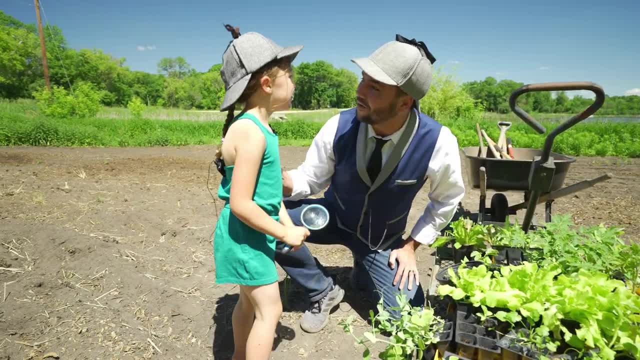 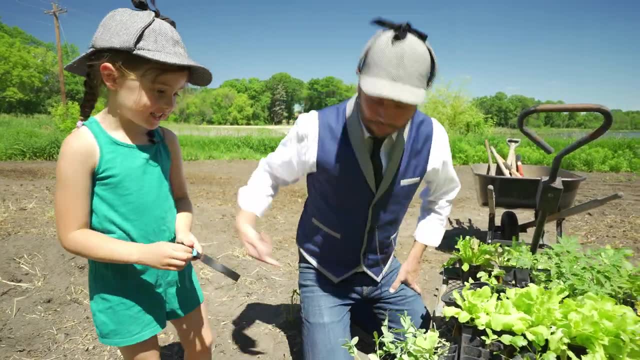 Piper, come here. Hi, Piper, How old are you? I'm half a year old. How old am I? I'm 30! Isn't that old? Yeah, Yeah, it's so old. Well, hey, look at all these plants, Piper. 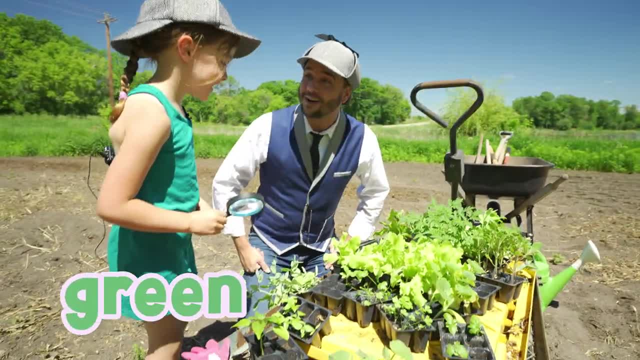 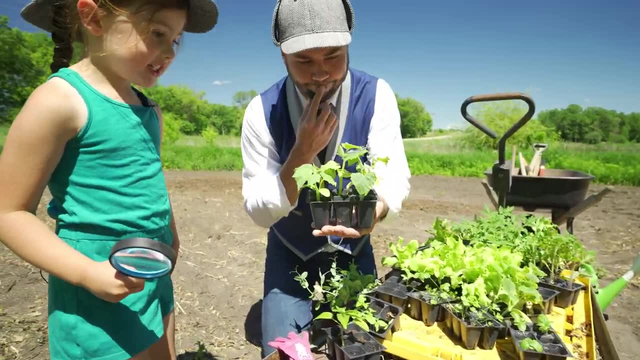 What color are they? Green. There's so much green. They're getting really big, aren't they? Yeah Well, let's see. what kind of plants do we have? What kind do you think this is Um cucumber? 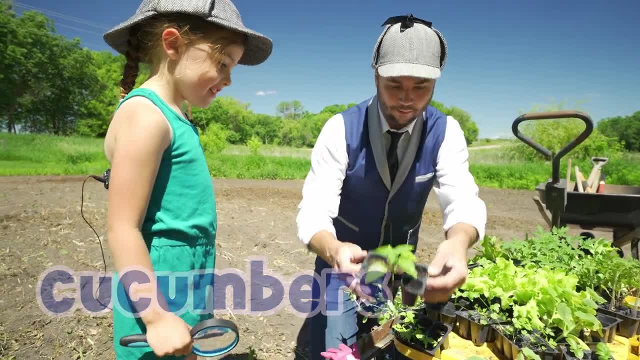 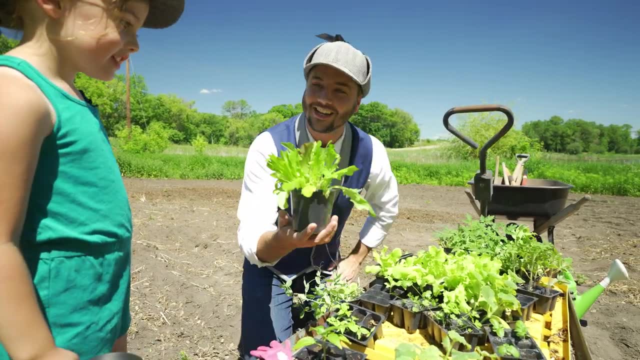 That's right, They're cucumbers. They're getting so big. What about this one, Rainbow bell pepper? Wow, they're going to be so colorful, aren't they? Yeah, Oh, look at this one. What do you think this is? 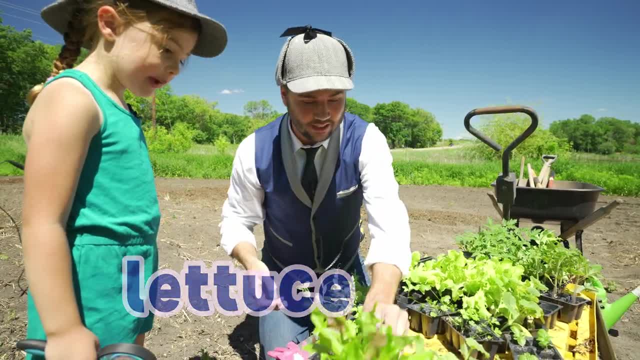 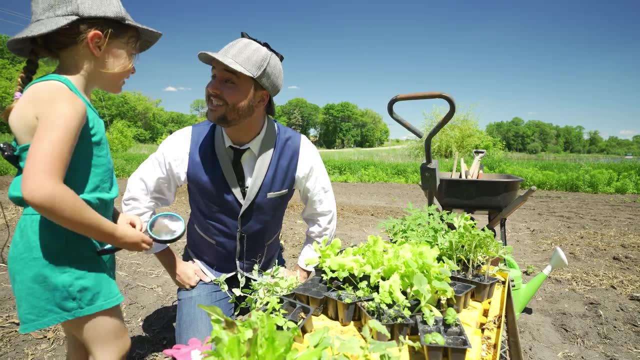 Lettuce, Lettuce. Wow, that's so awesome. We have so many different plants to put in the ground, don't we? Yeah, Hey, you know what would be fun? What if we took a dance break? Yeah, let's do it. Here we go. Come on, let's dance. 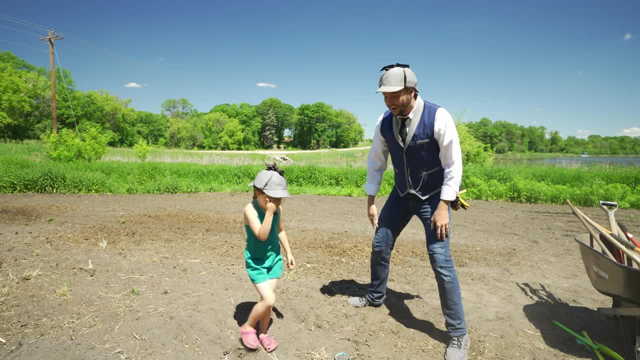 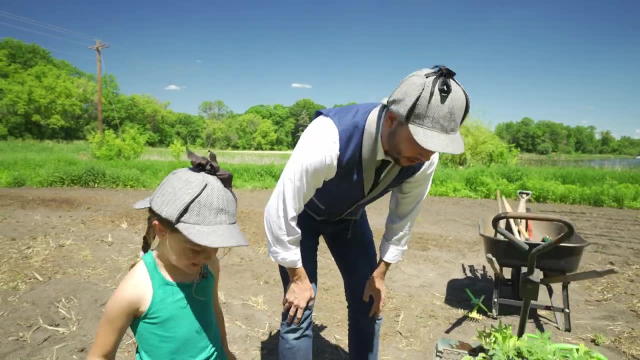 Wow, that was so much fun. Thank you for dancing with me, Piper, You have some great dance moves. Thanks, Hey. do you think we can start planting some plants now? Yeah, All right. well, before we start, we've got to get our gloves on. 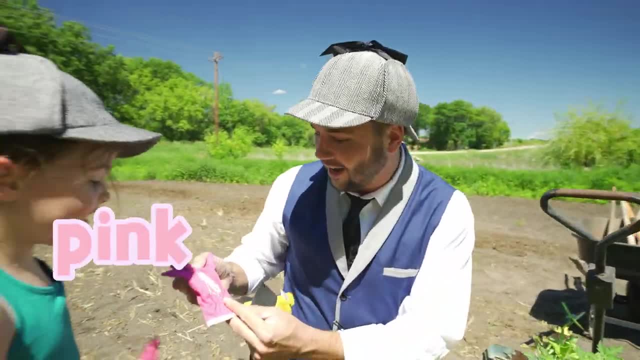 Yeah, Whoa. what color are your gloves? They're pink and there's a unicorn with a scooter And a unicorn. Do you think I could put these on my hands? No, No, they're a little too small, aren't they? 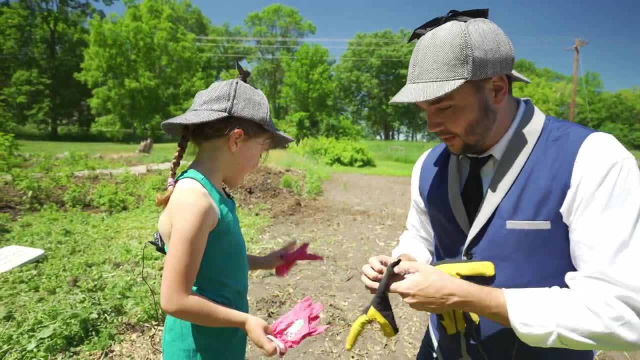 Yeah, Yeah, here you go. Why don't you put on yours? I can't, I can't do it, You can't do it. Well, here, how about I help you out? You ready, I'm going to go like that, Looking good. 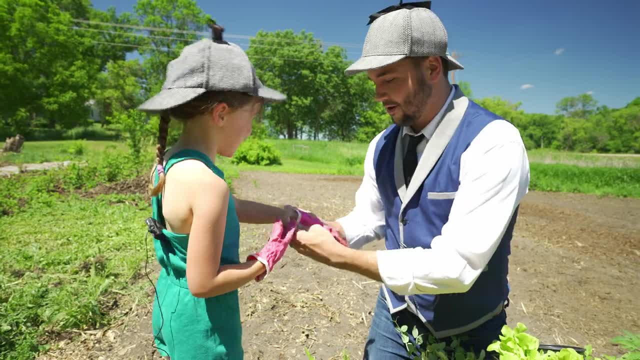 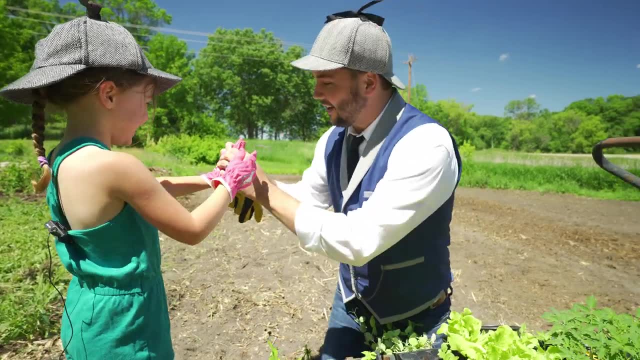 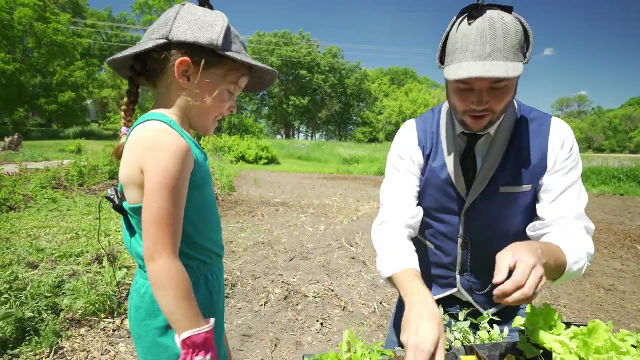 There, There's one. Oh no, There you go. Oh no, Oh no, Got it. There we go. All right, I'll put mine on. Do you think I can put mine on by myself? Yeah? 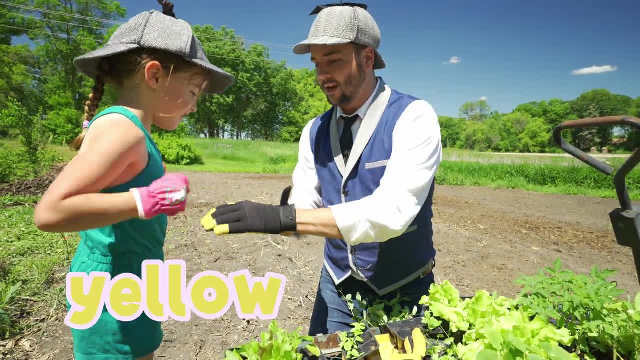 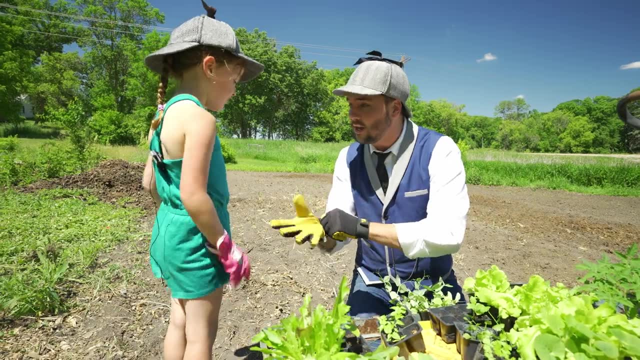 Yeah, I think so too. All right, here we go. What color are my gloves? What do you think? Yellow and black. Yellow and black. Great job, That's awesome. All right, so we've got our gloves on. Looking good, right. 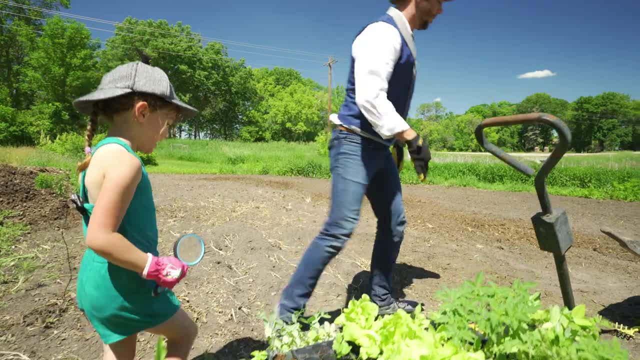 Yeah, Now let's go over and grab some tools. We've got to prepare the soil. Come here, Okay, All right, first thing we're going to need is a rake. I've got my rake. I have this one. 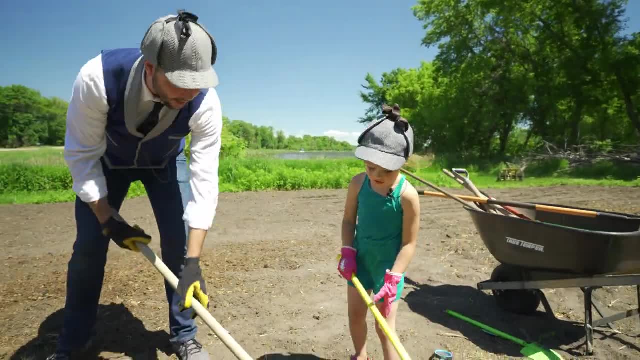 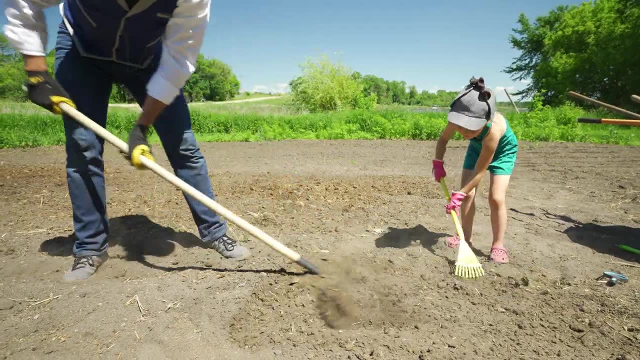 Look at that. All right, we're going to plant them right here. So let's take our rake. We're going to rake the ground. We want to get a nice and level ground for us to plant our seeds in. That's looking good. 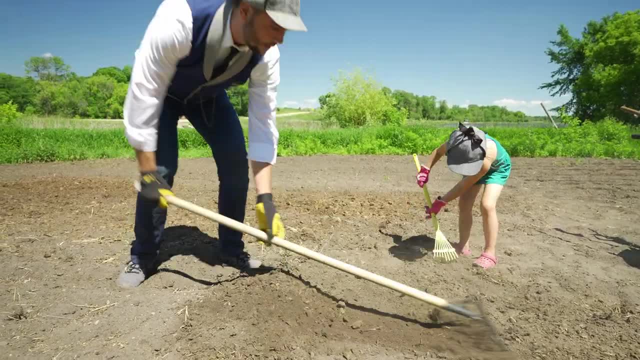 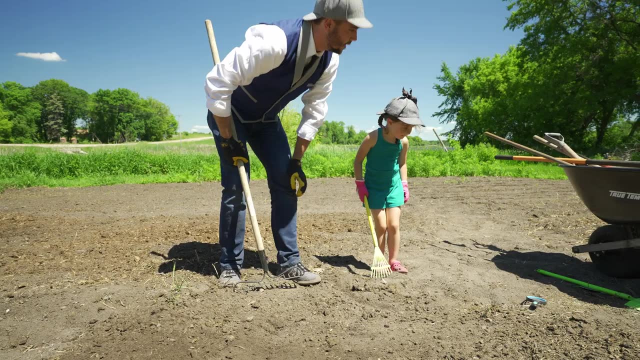 Great job, Piper. All right, There we go. We've got a nice flat level ground, so we'll plant some out here. All right, let's see. What tool do we need next? I think we need a hoe. I've got one of those. 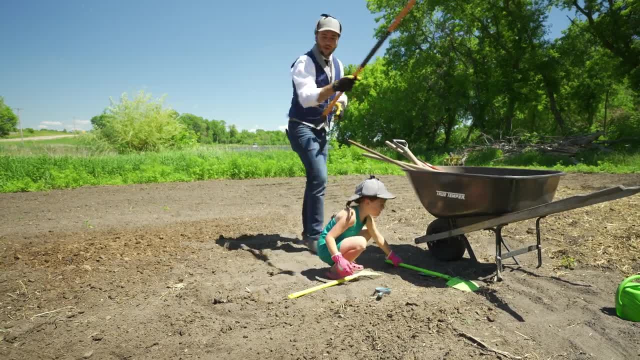 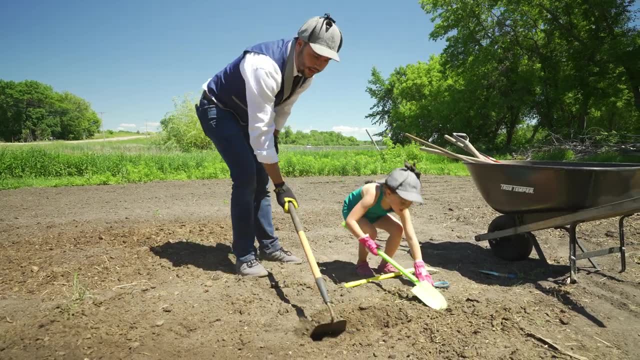 I don't have a hoe. You want to grab your shovel? Yeah, I'll do this one. Let's do that. All right, so we're going to make a little bit of a trench. I'll do it like this. That's great: A little bit of a trench. 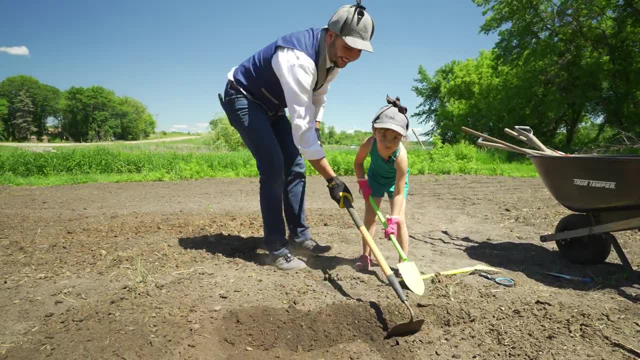 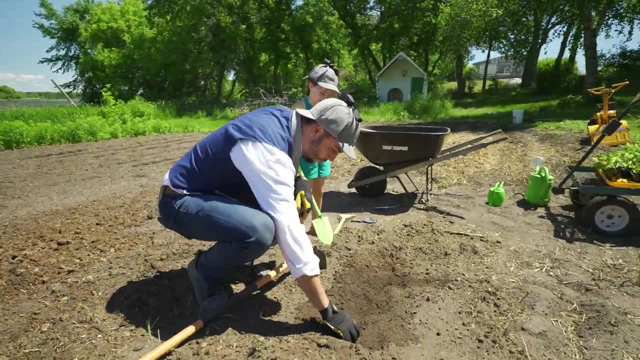 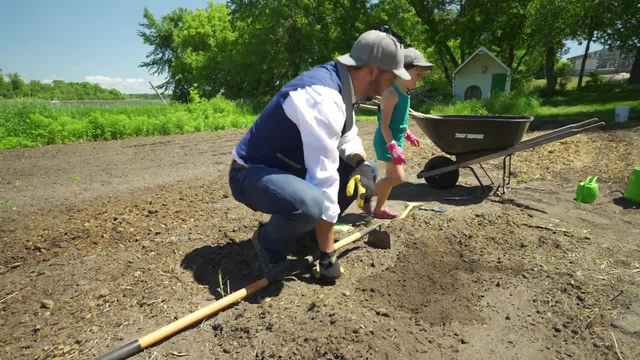 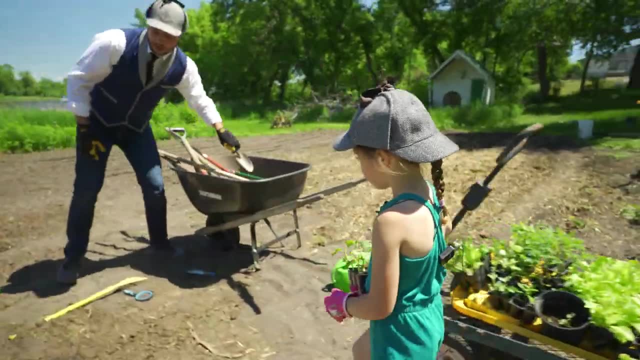 Hey, do you think you could go grab the cucumber plant? Yeah, Yeah, Let's get the cucumber plant. Great job, Piper. All right, first thing we'll plant is cucumber. So we've got our little shovel and you've got one too. 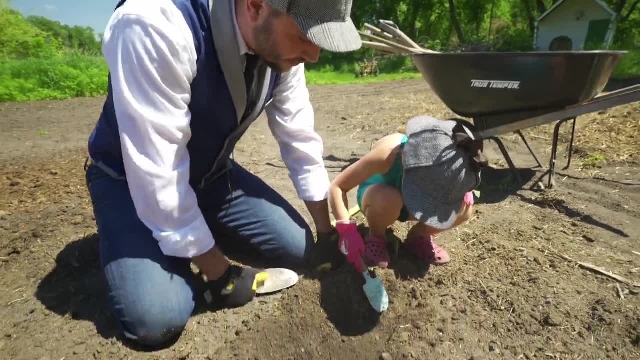 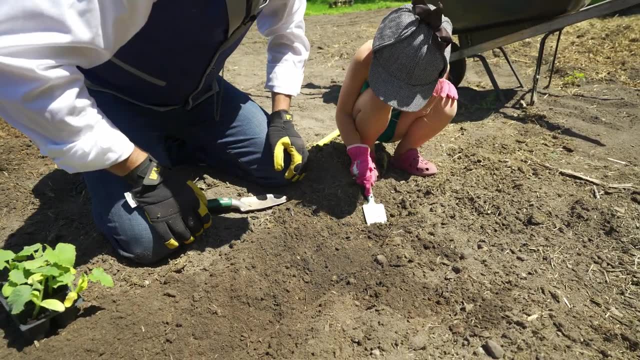 Yeah, it's a blue. Let's start digging a hole right there. Do you see all the ants? Yeah, Oh, there are so many of them. I know That's so funny. Look, there's one down there, Whoa. 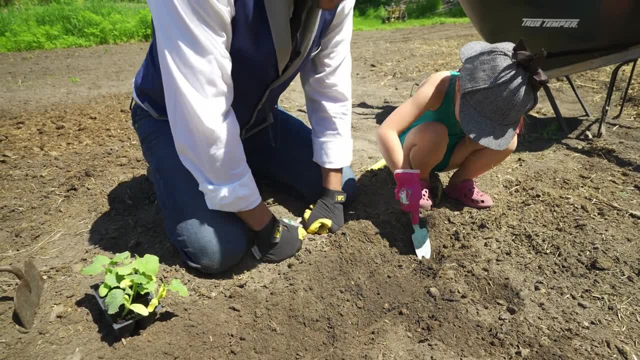 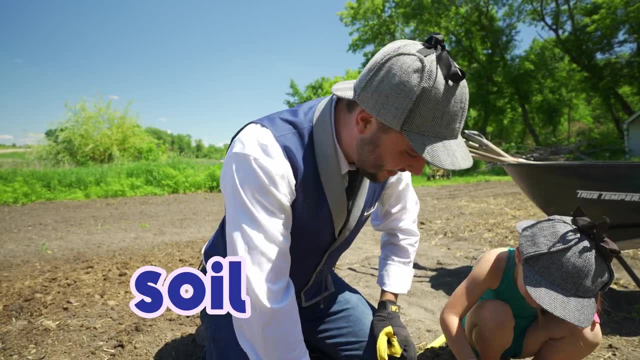 That's right. All right, you keep digging, Keep digging, Looking good. So remember, plants need three things, and the first thing they need is soil. Yeah, That's another word for dirt, Mm-hmm. So we're going to put it in the dirt. The second thing it needs is sun. 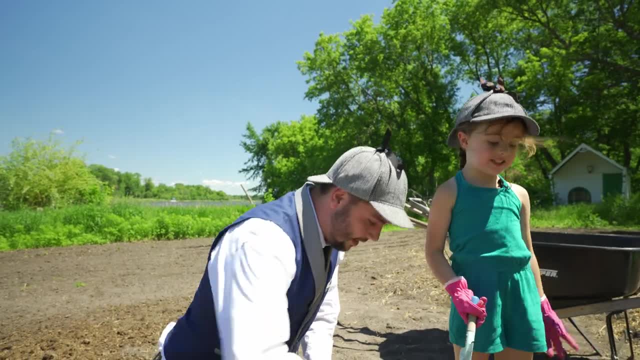 Mm. Thankfully, it's really sunny out, isn't it? Yes, It's a little cold. It's a little cold, Mm-hmm. Well, maybe you should try wearing long sleeves. All right, here we go. 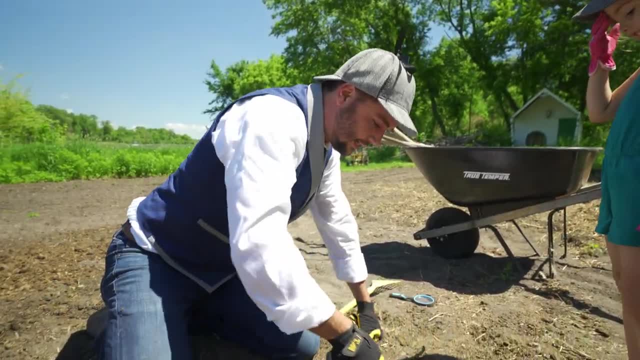 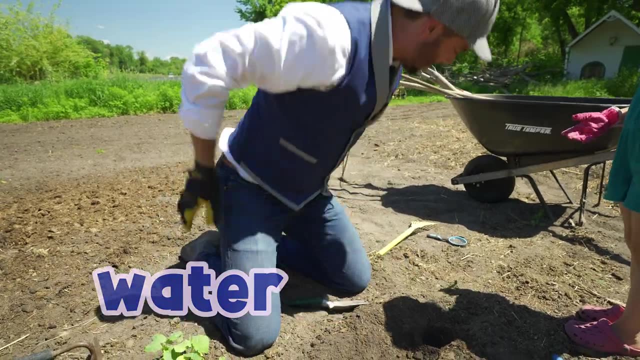 No, it's hot out. It is hot out. All right, we're going to dig this down. The third thing that these plants are going to need is water. Yeah, So we'll make sure that they have water. All right, look at this, Piper. Why don't you grab a magnifying glass? Let's inspect this. Look at that hole. 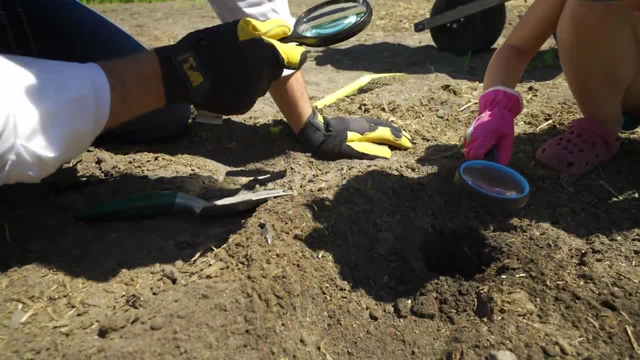 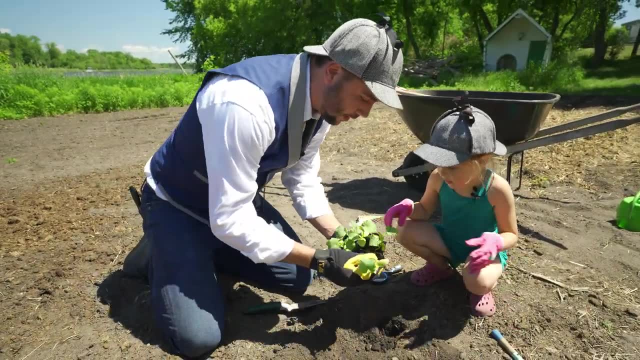 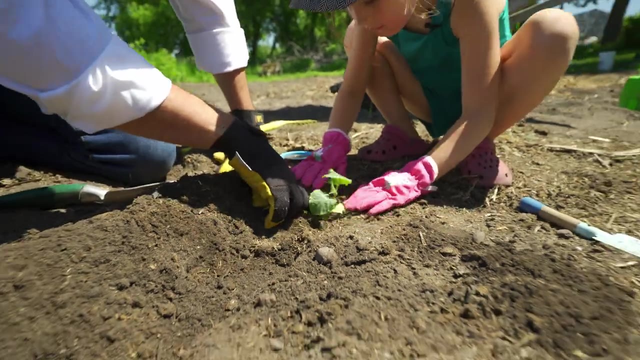 Ooh, You think it's ready for the plant now? Yeah, I think so too. Here we'll put one of these in, So we're just going to gently pull it out And we're going to put that in. Great job, That's looking good And we'll fill in the dirt around it. pat it nice and tight. Look at that. We planted our first cucumber plant. 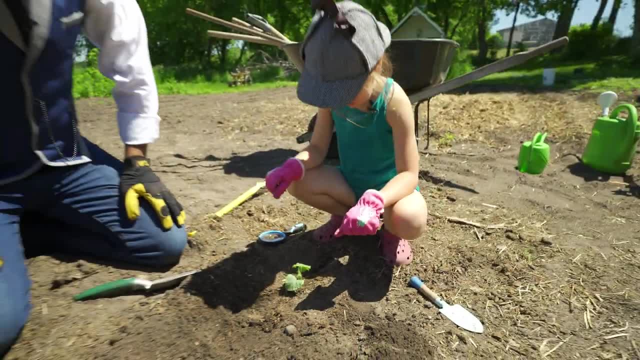 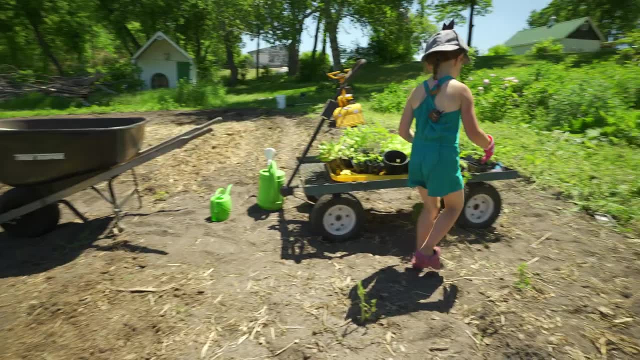 Ooh, Great job, Piper. Which one should we plant next? The rainbow bell peppers. Yeah, Why don't you go grab the rainbow bell peppers? There's only one of them, That's right, So we will plant that one, All right. 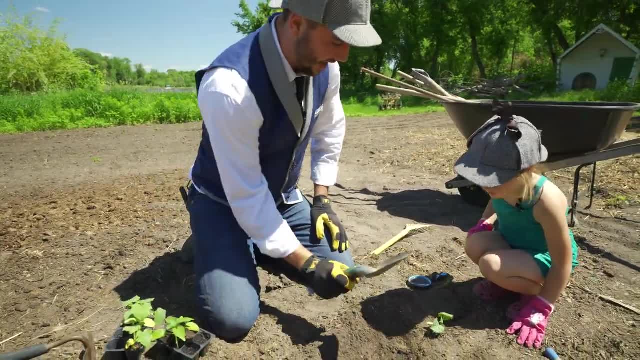 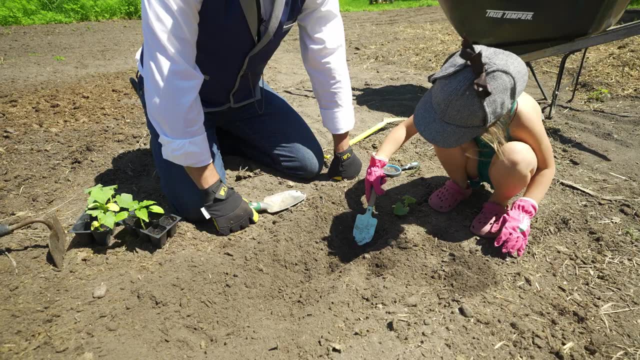 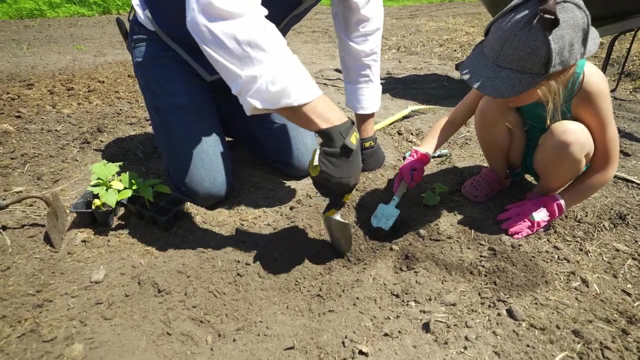 So what do we have to do next? Get another shovel and dig another hole, That's right. So let's dig it right around here. There you go, Looking good, Looking good. There's no ants in this one, No ants in that one. Here, let's dig a little farther over. Let's go right here. 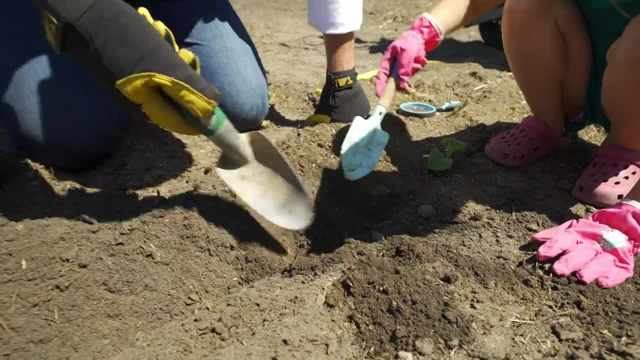 Yeah, Let's dig right there. I'll do the first scoop. There we go. You want to get some more? I need an even bigger scoop. That's right, You got an even bigger one. Here we go, Let's open that up. I'll get a couple more scoops. 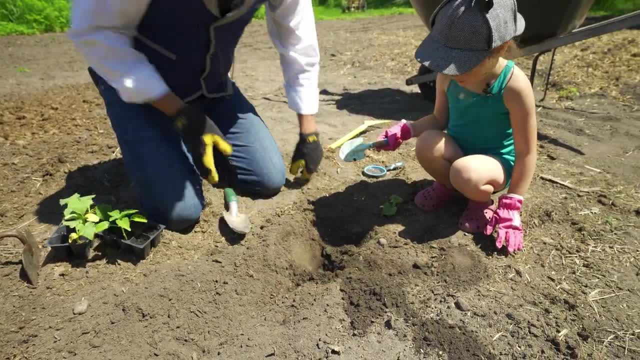 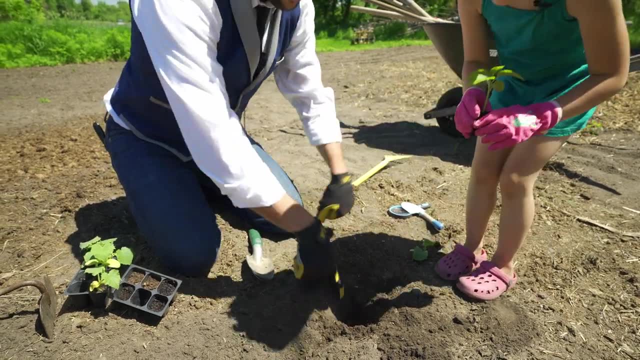 Okay, All righty, Now we're ready to plant the rainbow bell pepper. Oh, it's so windy. It is windy. Do you want to put this one in here? Yeah, Very gentle, Very careful, Let's get that in the hole. Excellent, Excellent. Now let's put some dirt around it. 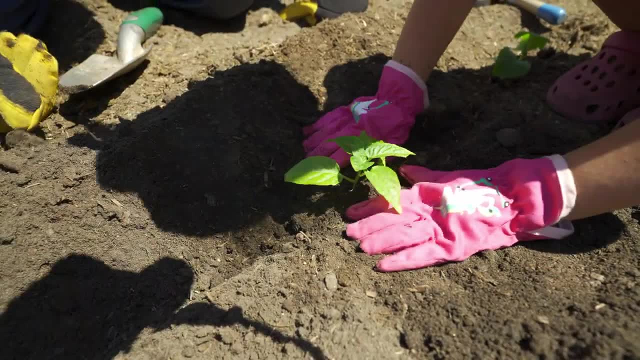 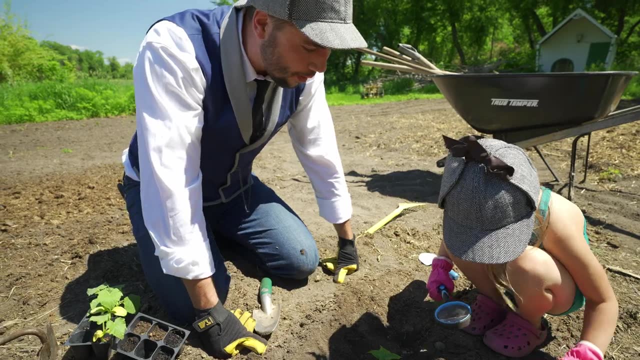 Oh, that's looking great. That's super good for the rainbow bell pepper. Yeah, Wow, Hey, do you think we could get one more planted? What's our last one? Lettuce, Lettuce, That's right. 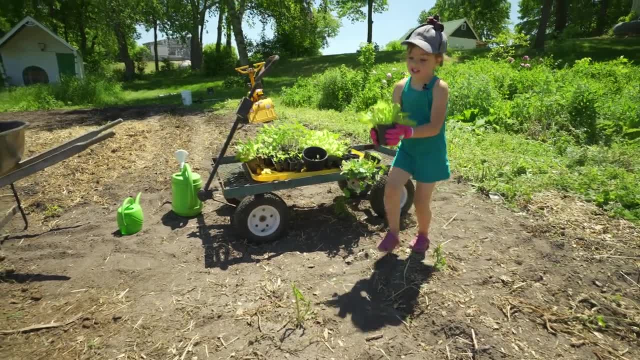 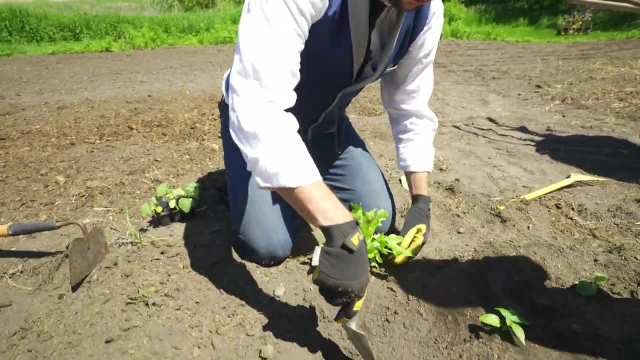 There's so many. Yeah, There's so many of it. There's a lot. It's really big, isn't it? Yeah, It's even bigger. That's right. We're going to have to dig a bigger hole. Let's dig it right over here, Piper. 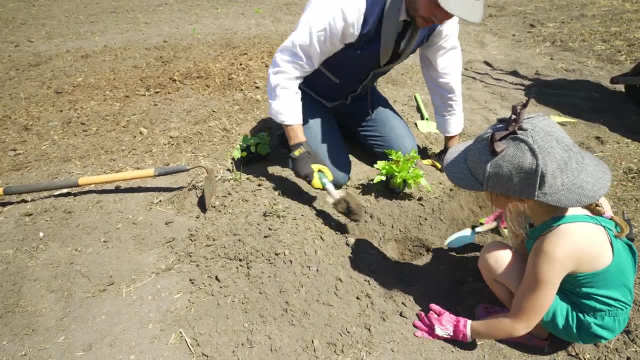 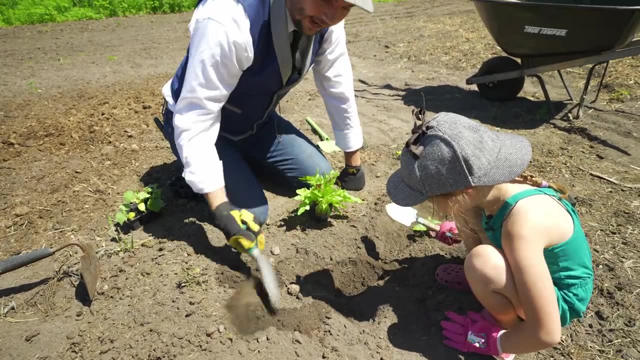 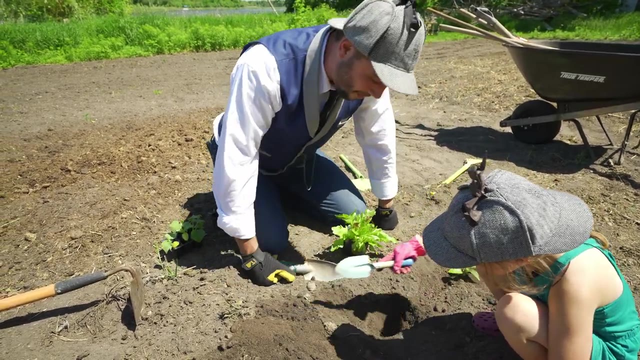 Okay, Ready, I'll get the first dig. I'll do a huge one. Let's see a big one. Wow, That was great. All right, I'll do the next one. You ready? There you go, Looking good, The plant is pretty big, so we need a big hole. 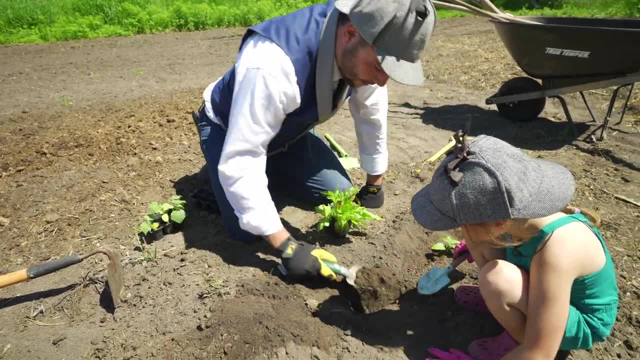 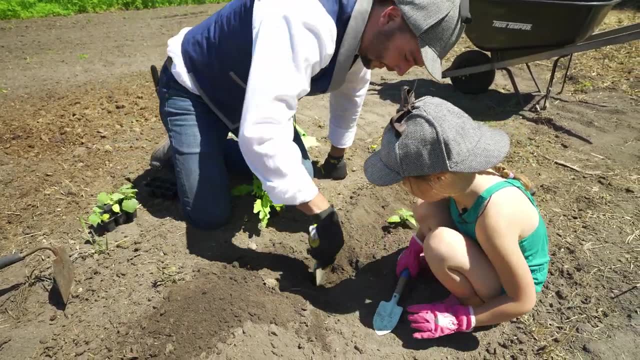 Yeah, All right, We'll get another scoop in here. That's good, That's good. Do you think that'll fit? No, Let's do it a little bit deeper. How about a little bit deeper? Here we go, Yeah. 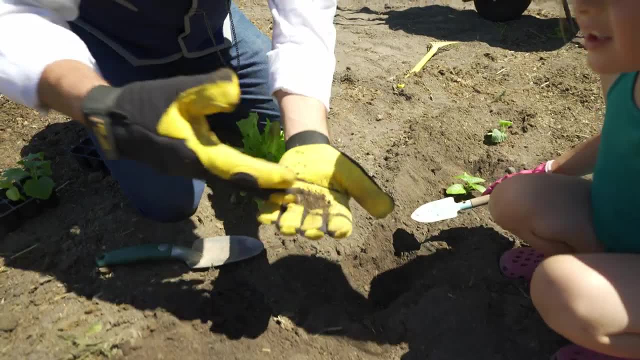 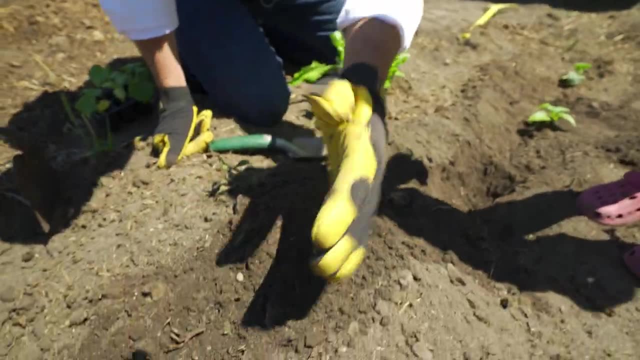 Hey, look at this. I think we found a worm. Wow, Wow, How cool. is that So cool? We found a worm. All right, We'll put him down right there. You can stay there, Mr Worm. All right, Piper, Are you ready to put the lettuce plants in? 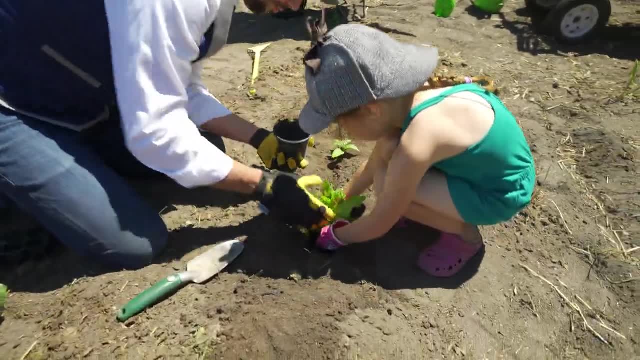 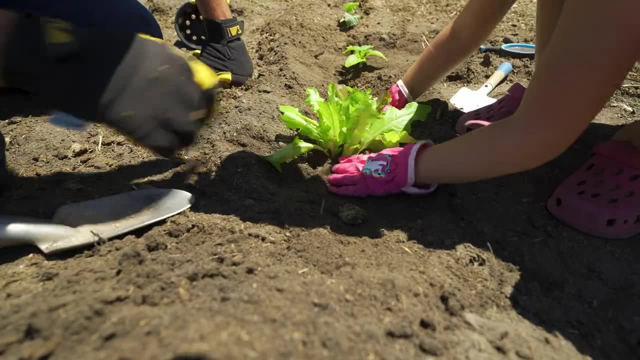 Yeah, All right, Here we go. Very gentle, Very gentle, Put it down, Excellent, And we'll fill it in with some dirt. I just saw an ant go there. An ant, No way. Yeah, All right, We'll settle that in. How does that look, Piper? 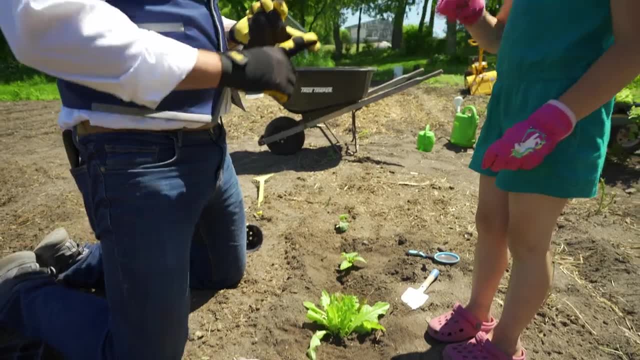 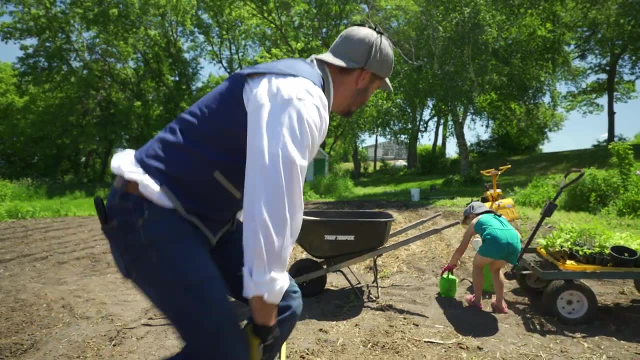 Good, That looks so awesome. All right, So we've got the soil, We've got the sun. What was the last thing that they need? Water, Water. Hey, let's grab our watering cans. I have this little one. 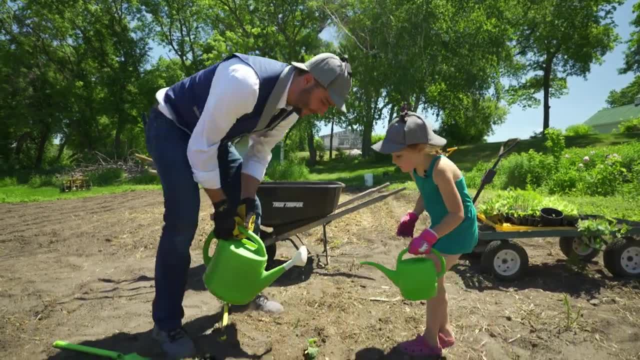 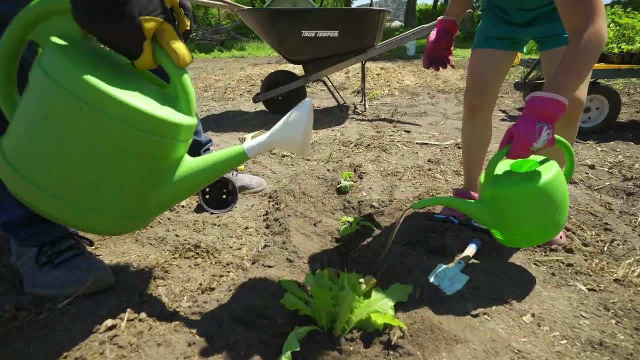 Yes, you do. I've got a bigger one You ready. Let's water the plants. I'll water the rainbow belt plants. That's a great idea. I'm going to water the lettuce one And then put a little bit on the lettuce. 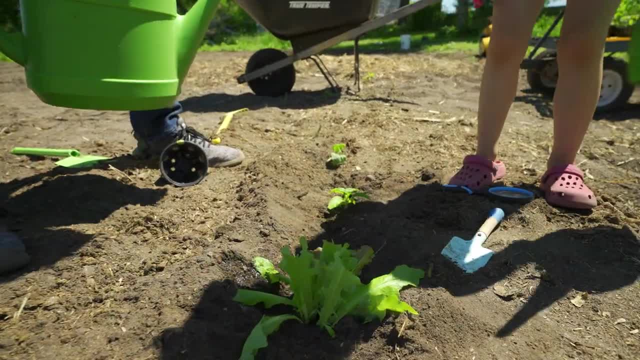 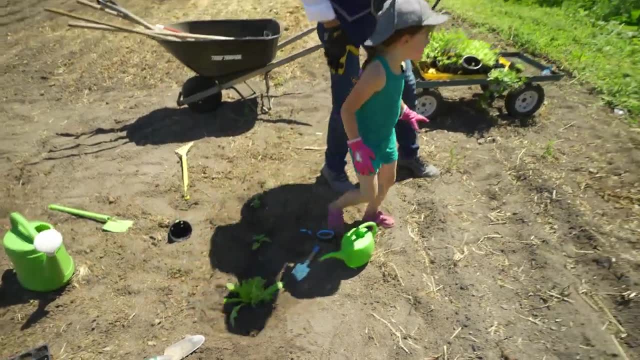 There we go. Oh, that's looking great. Wow, I can't wait to see the plants that we get. Well, hey, let's come look over here, Piper. Let's go explore some of the rest of the garden. We can check out what we have growing. 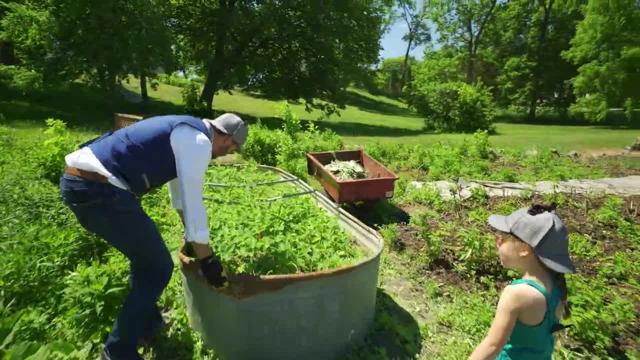 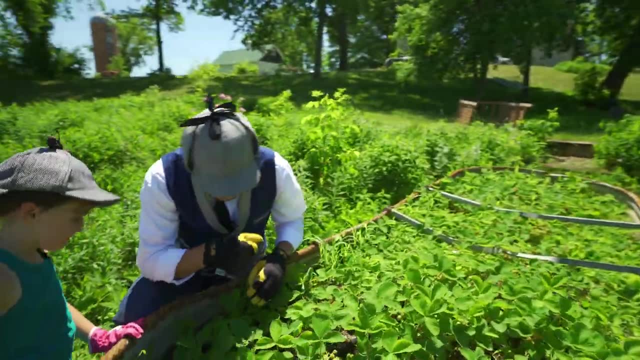 Yeah, Oh, wow. Look at this, Piper. Do you know what these are? Strawberries, Strawberries. I love strawberries Really. Yeah, they're so juicy, So juicy and delicious. I had some for breakfast today, Did you? 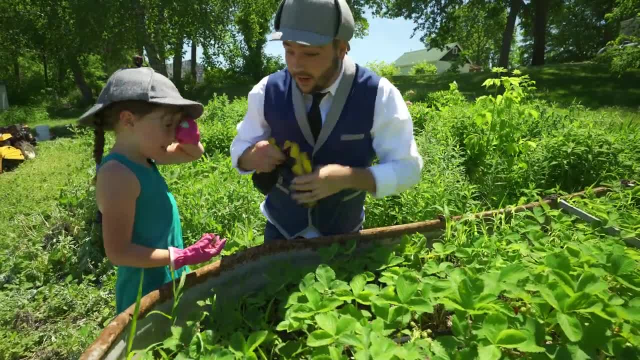 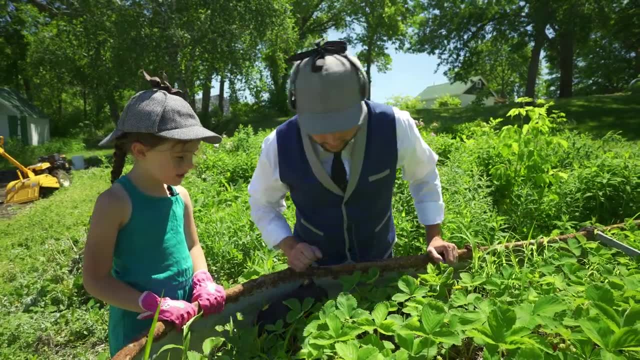 Really, Yeah, No way. I had some pancakes, Chocolate chip pancakes, Chocolate chip pancakes. I love chocolate chip pancakes. Did you have syrup on them? Yeah, Yeah, I love syrup. Well, hey, do you think we can find a red strawberry in here?